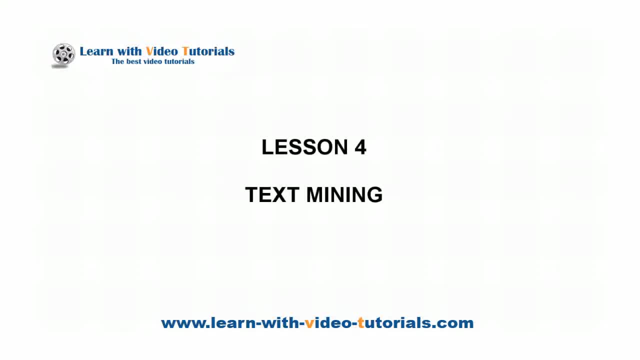 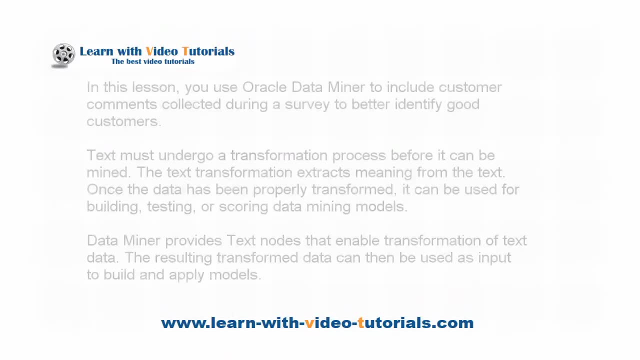 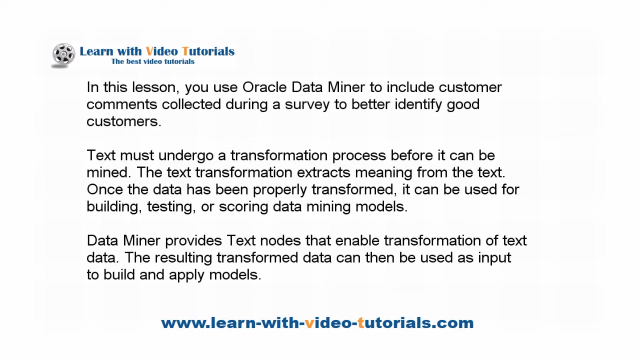 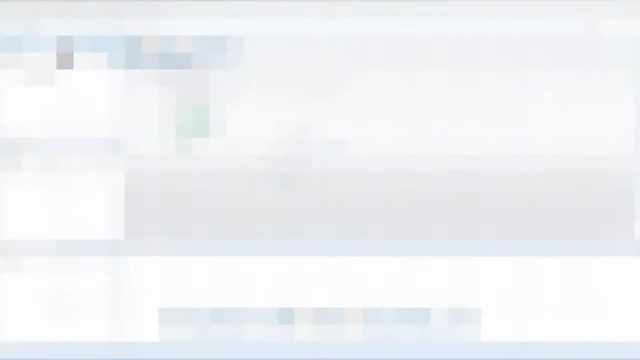 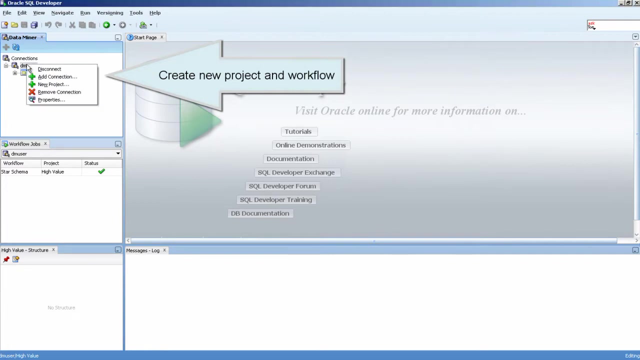 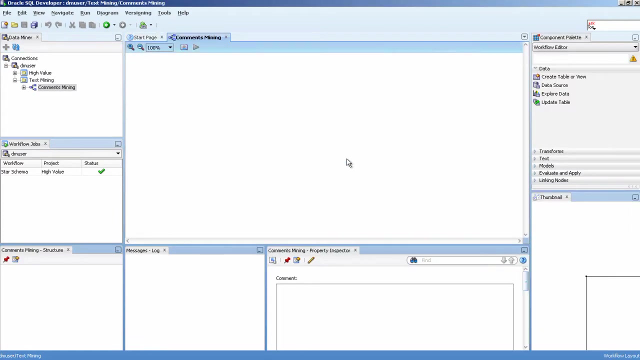 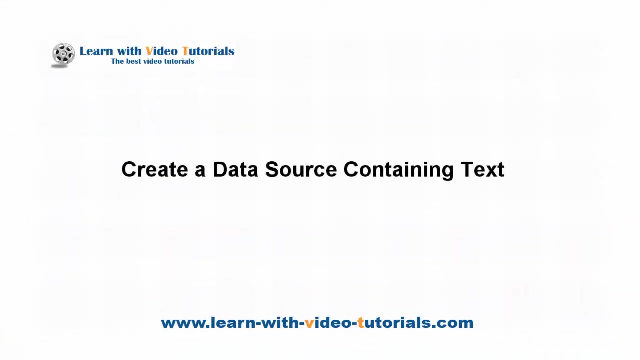 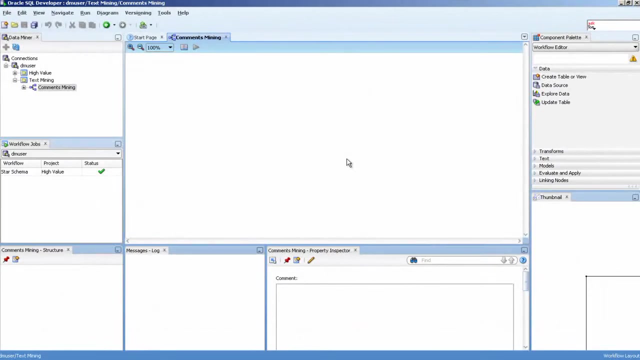 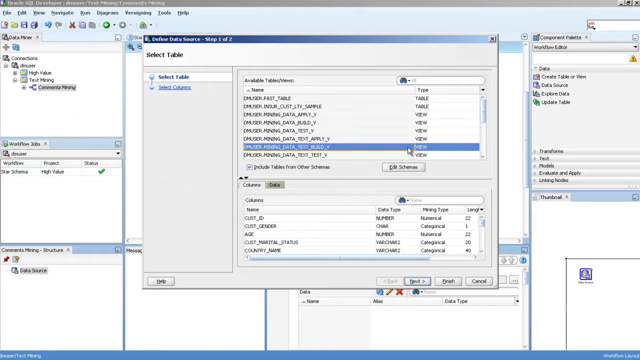 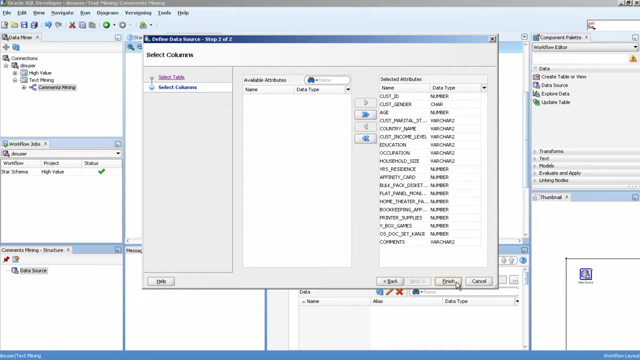 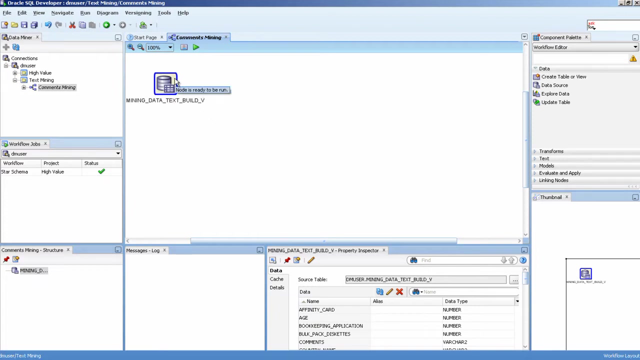 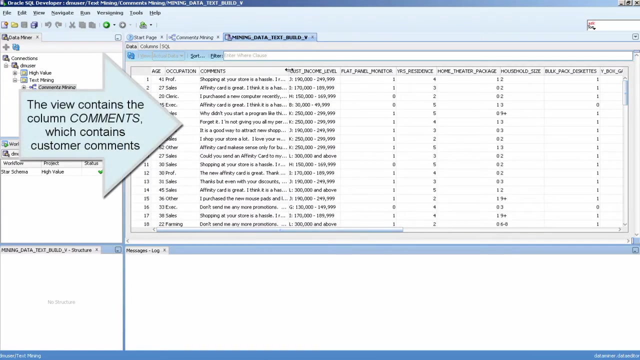 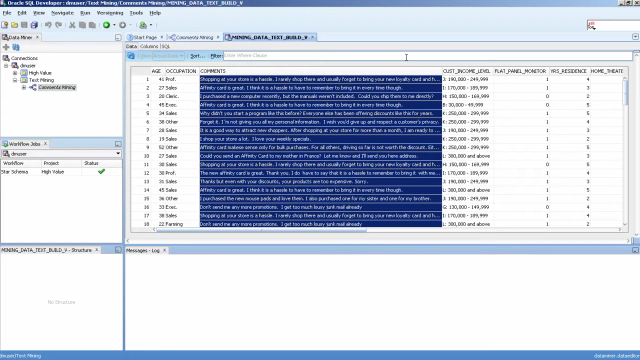 Lesson 4, Text Mining: Create new project and workflow. Create a data source containing text. Add a data source node to the workflow. Select the mining data text. build view. The view contains the column comments, which contains customer comments. Create a new layout to add new content. 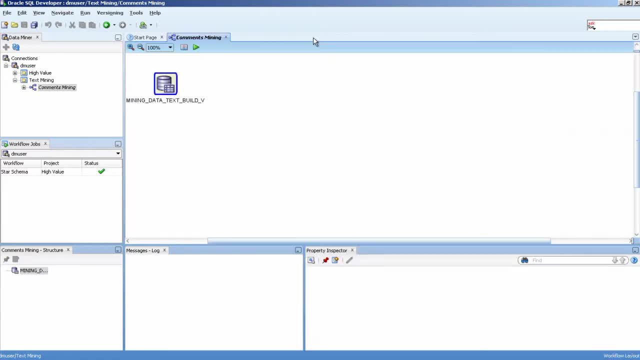 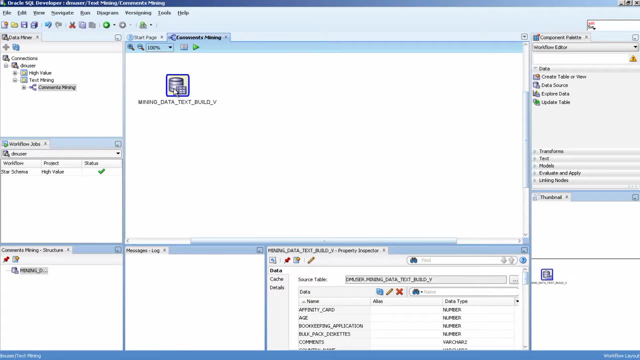 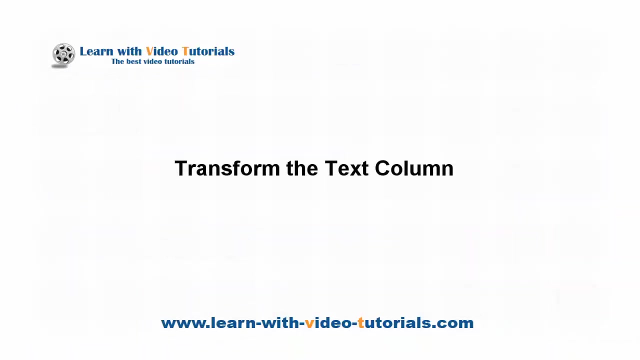 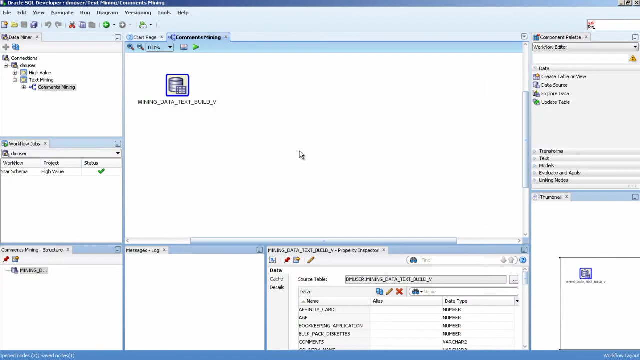 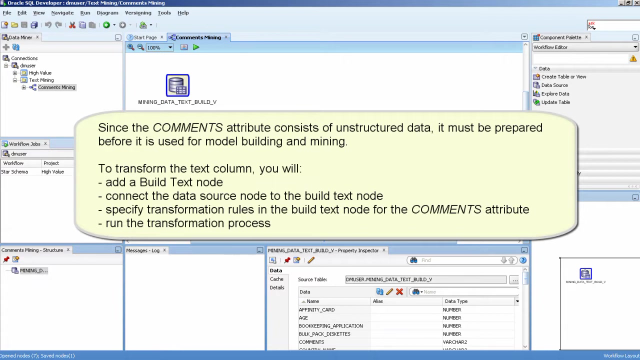 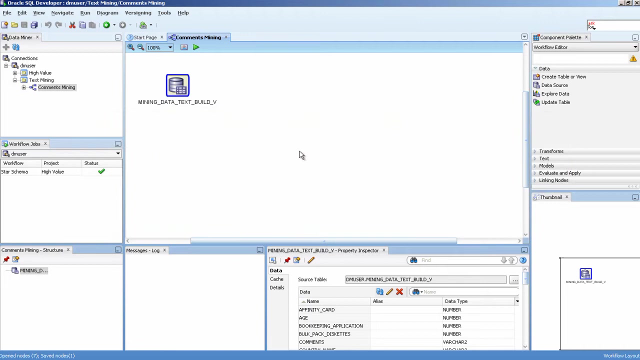 Create a new project. Choose the folder name. Select the plugin. Create a new plugin. Select the plugin. Create a new plugin. Create a new plugin. Create a new plugin. Transform the text column. Create a build text node. Change the node name to prepare build. 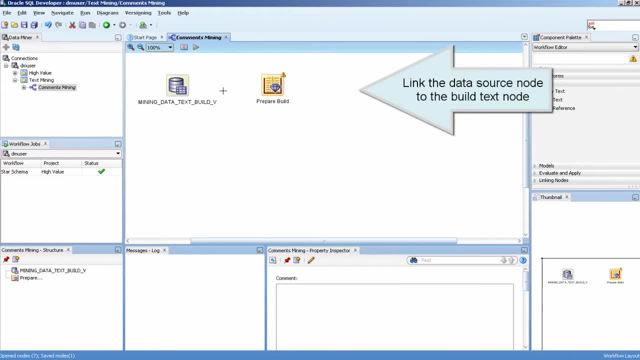 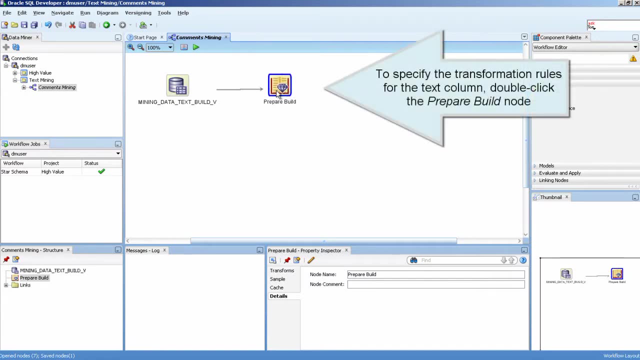 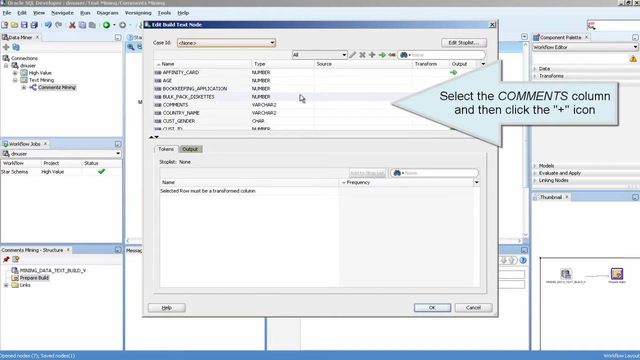 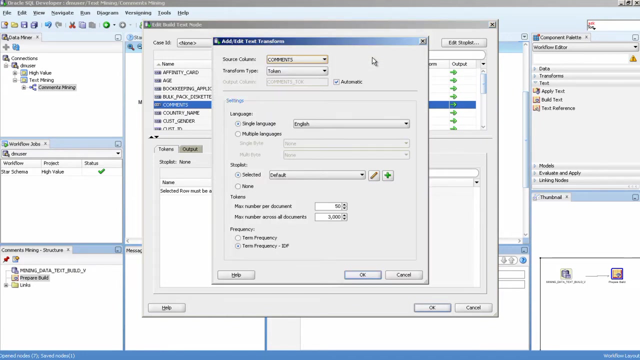 Link the data source node to the build text node. To specify the transformation rules for the text column, double-click the prepare build node, Select the comments column and then click the plus icon. Accept all of the default settings for the token type and click OK. 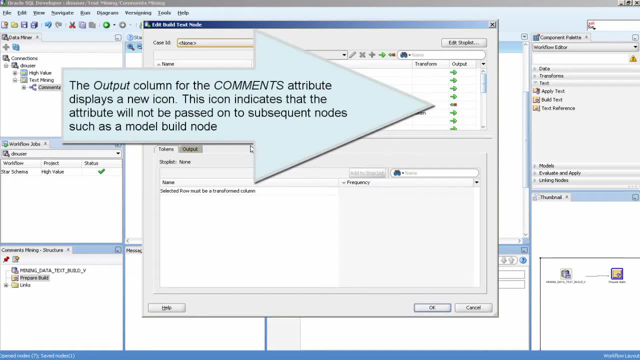 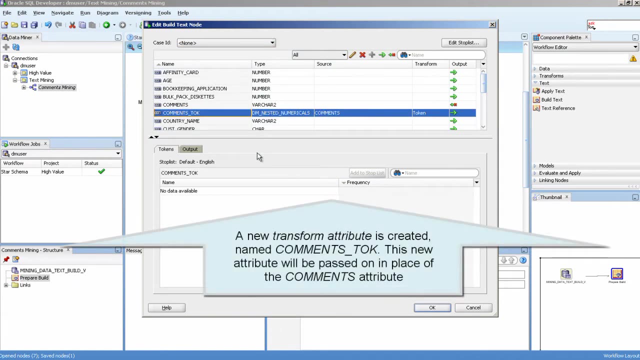 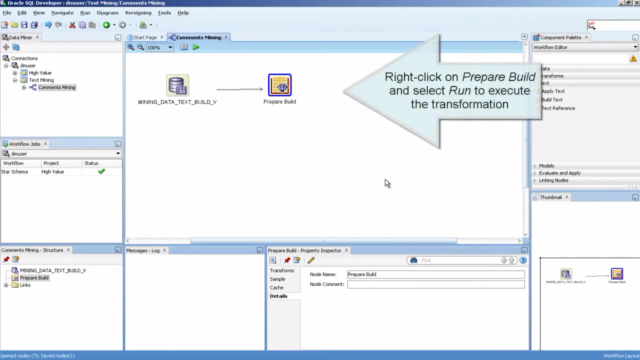 The output column for the comments attribute Displays a new icon. This icon indicates that the attribute will not be passed on to subsequent nodes, such as a model build node. Right-click on prepare, build And select run to execute the transformation. Double-click prepare, build and select comments stock. 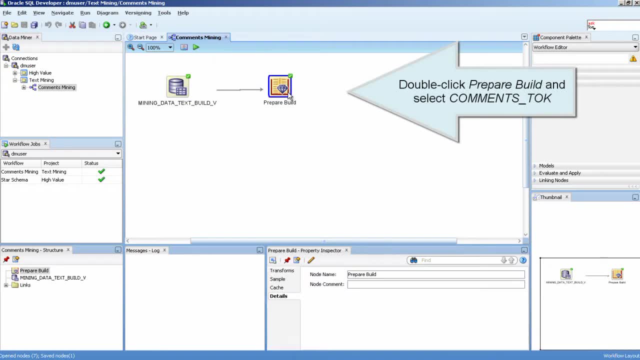 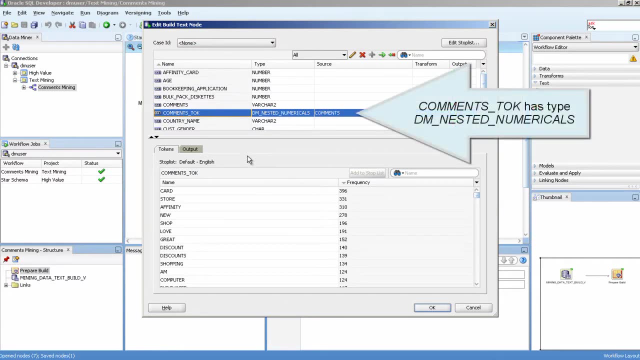 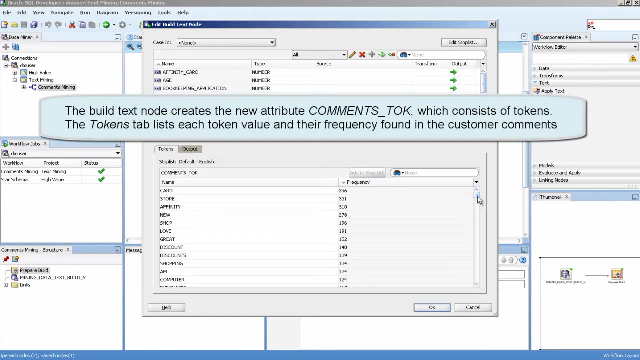 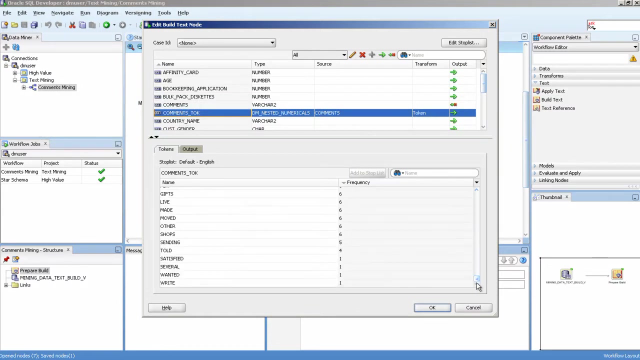 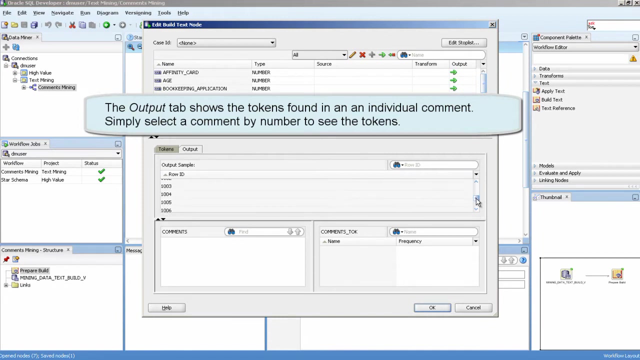 Double-click prepare, build and select comments. stock. The function will be verified and show that the changes are done. The project is now ready to use the software. If necessary, you can update the user profile by clicking on the sorry button at the end of the video. 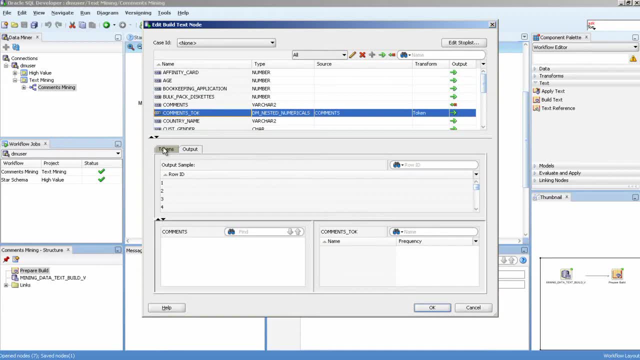 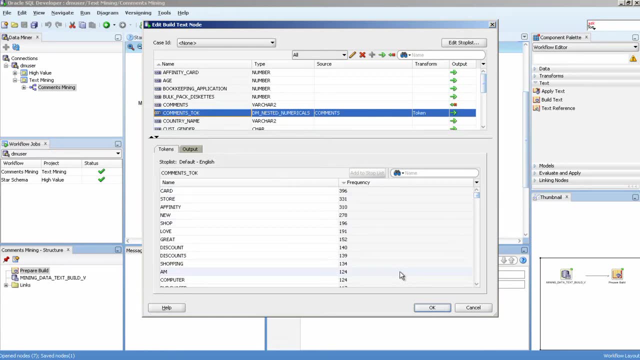 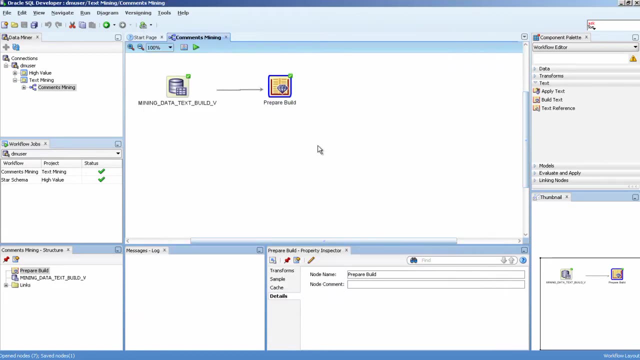 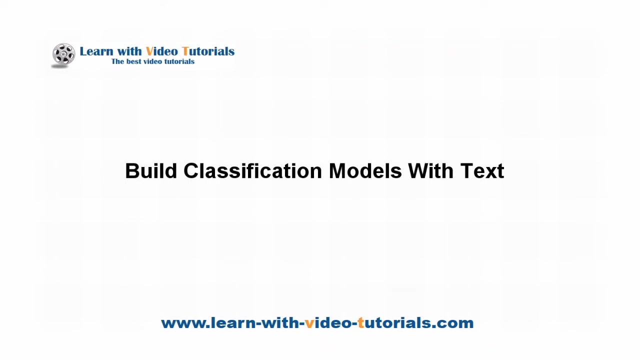 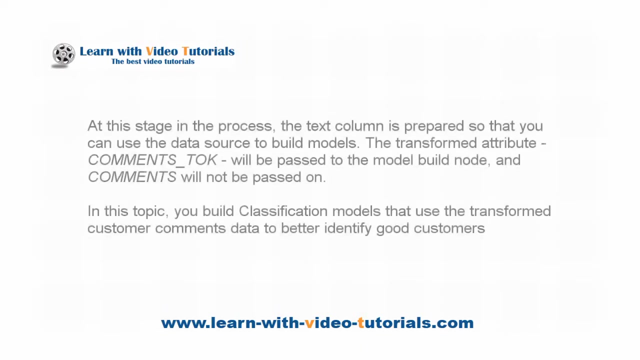 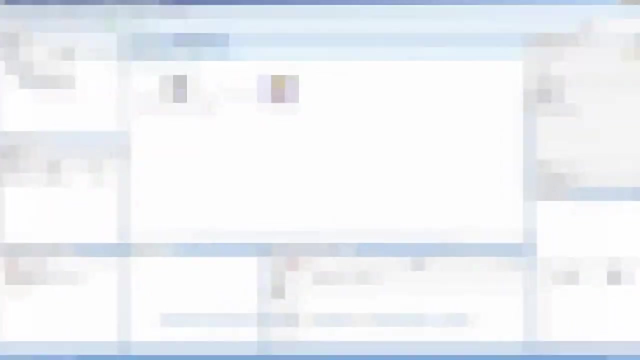 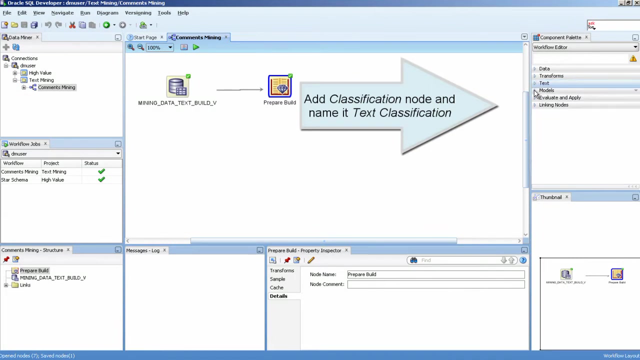 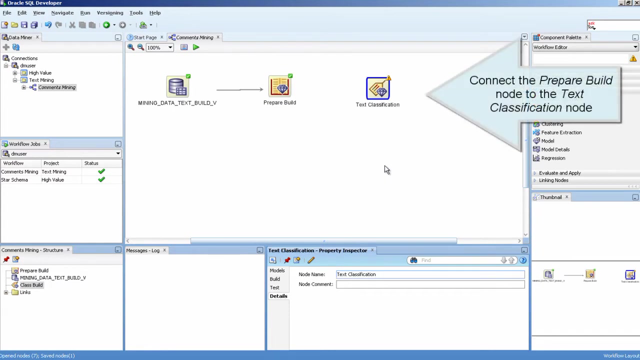 To enter the app password you must enter a code. This will automatically activate the auto-sync browser. Build classification models with text. Add classification node and name it Text Classification- buried classification data will appear. Connect the Prepare Build node to the Text Classification node. 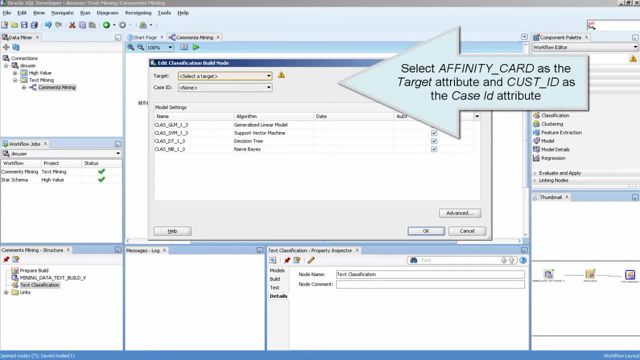 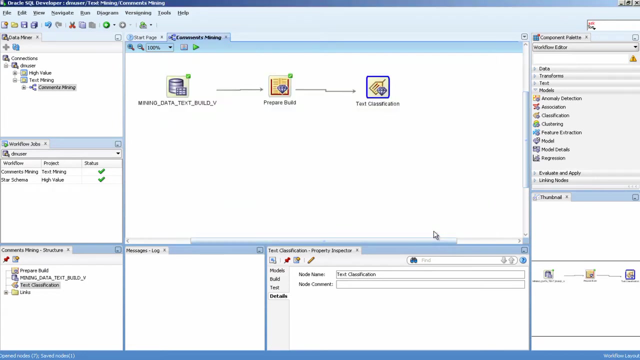 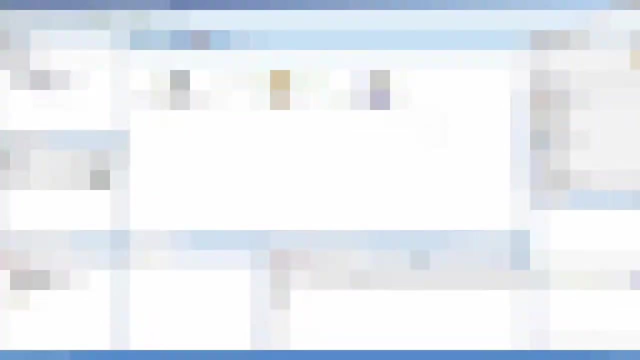 Create Affinity Card as the Target attribute and Cust ID as the KSID attribute. Run the node For tens of thousands of requests. click on Send. The box on the right shows the Chinese characters and the target class. Click on the Text Classified node to change the class. 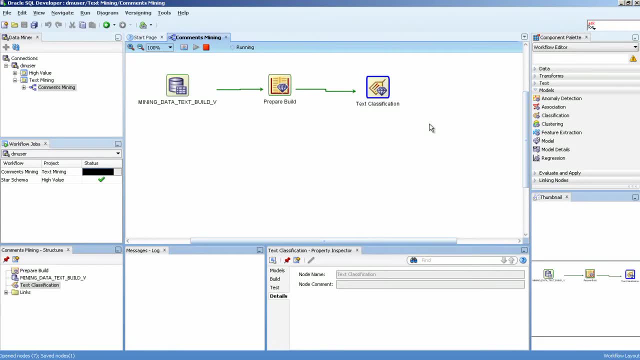 The box will show the current class number in the field. Click on the Text Classified node. Click on the Text Classified node again. The box will show the new class number of the time frame in the field. Click on the Text Classified node to save the standards. 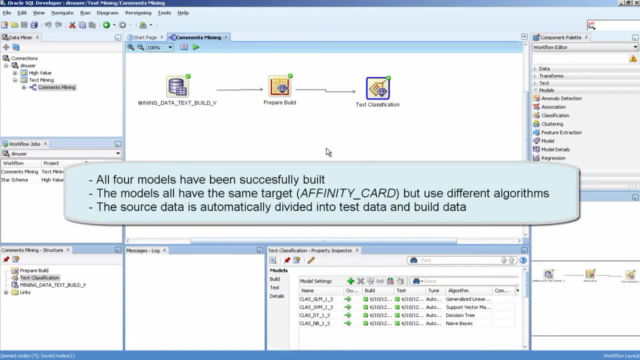 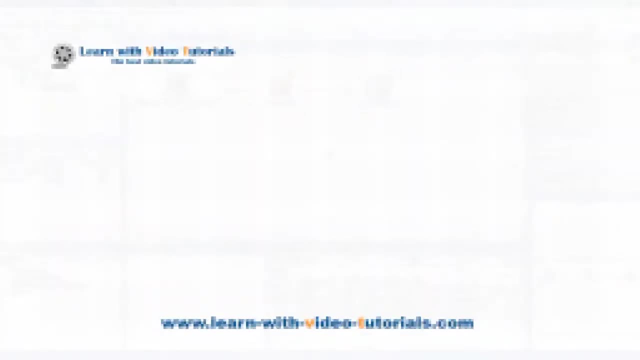 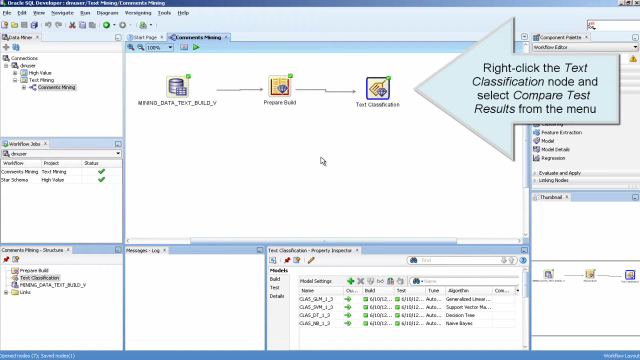 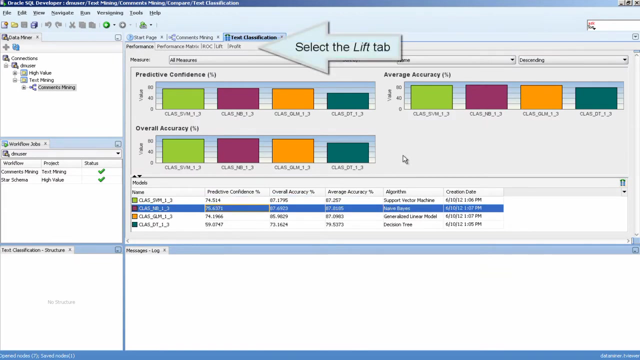 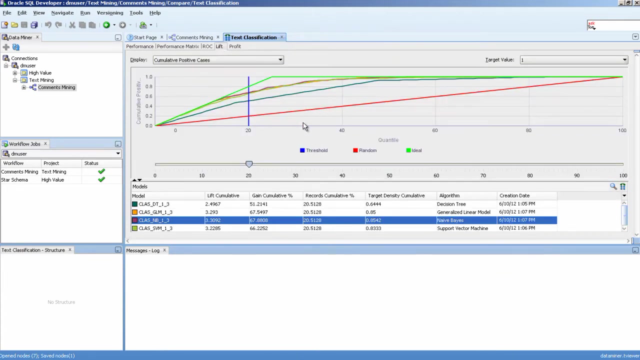 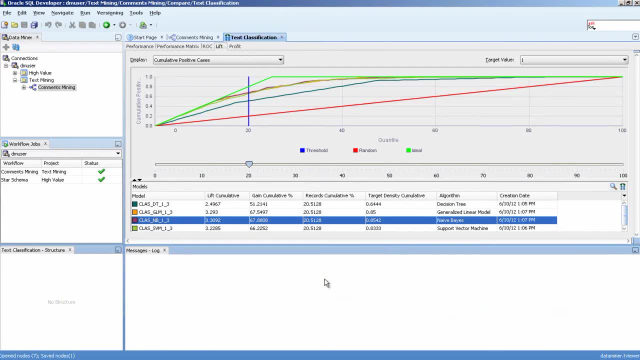 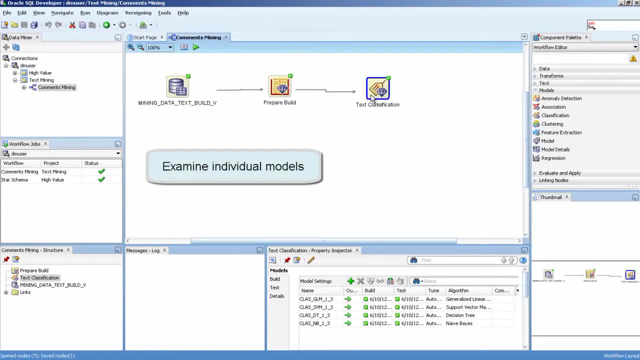 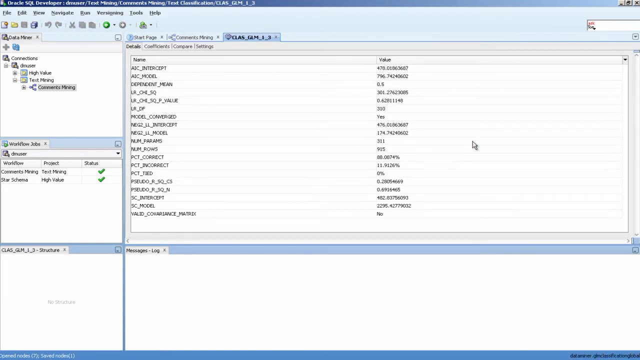 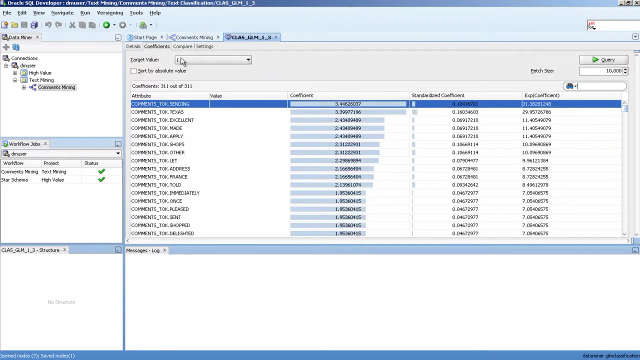 Examine the création status. Examine individual models: Model details. Model details: GAF-FGirls-Anesics-Jerking- incomers. Select the Coefficients tab to show coefficients for the tokens in the comment stock attribute. View the coefficient data for the SVM model. 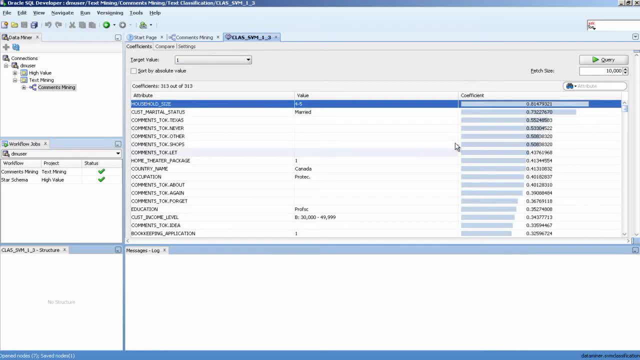 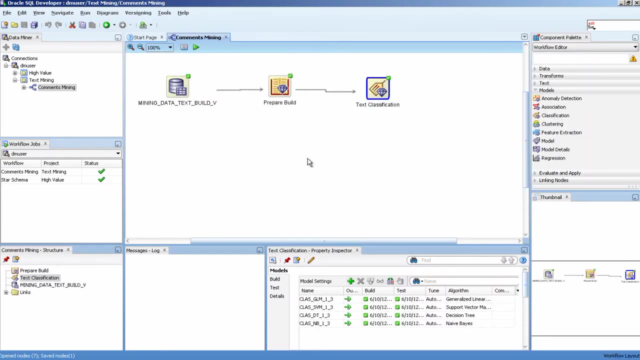 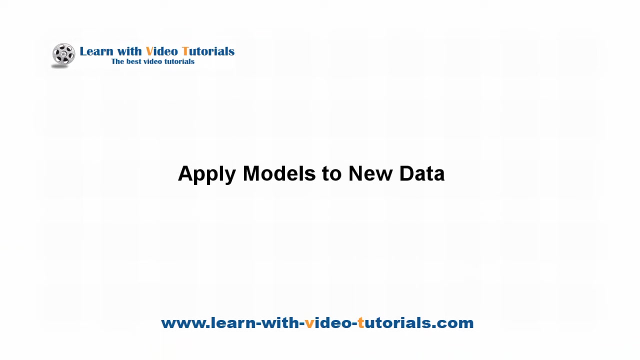 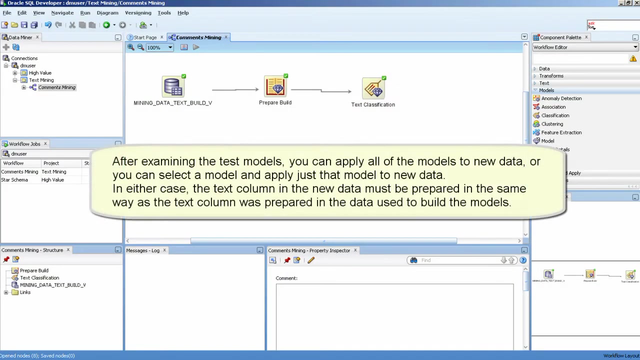 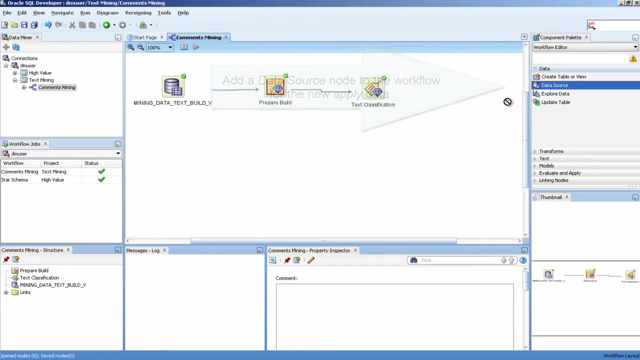 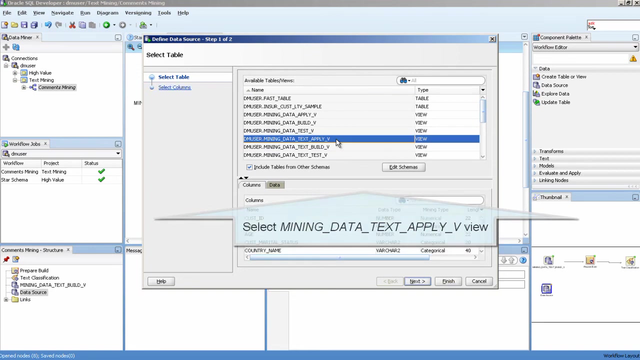 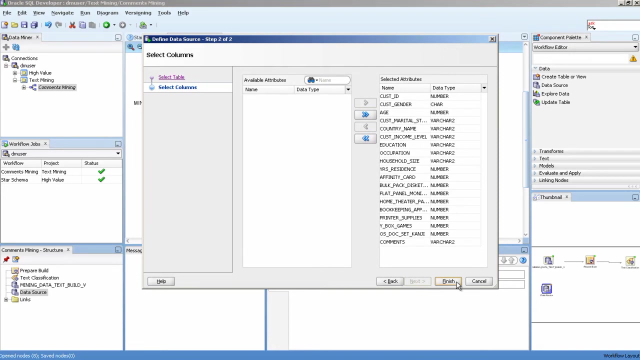 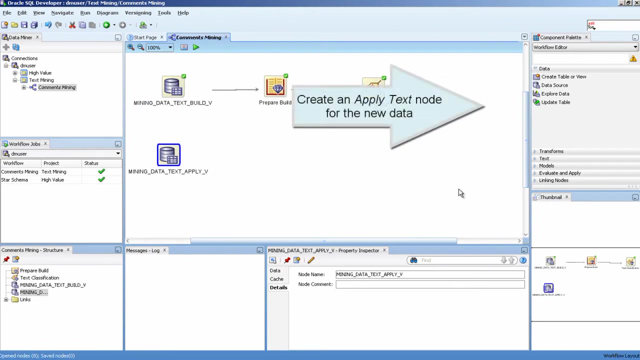 Apply models to new data. Add a data source node to the workflow for the new applied data. Select Mining Data Text: Apply view. Create an Apply Text node for the new data. Rename the Apply Text node to prepare- apply. Connect Mining Data Text Apply node to the Prepare Apply node. 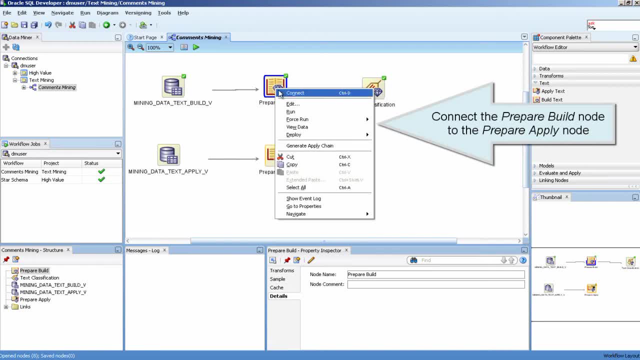 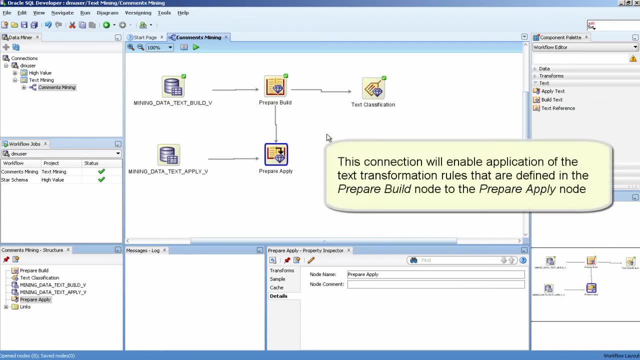 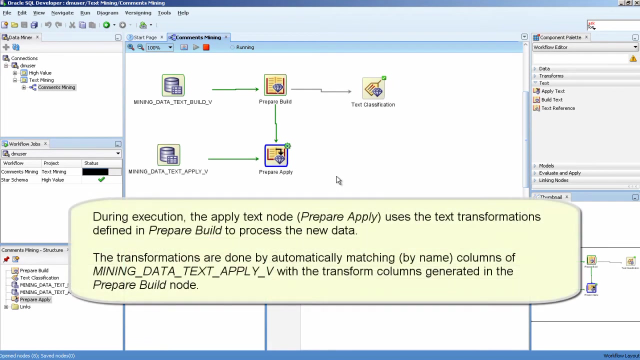 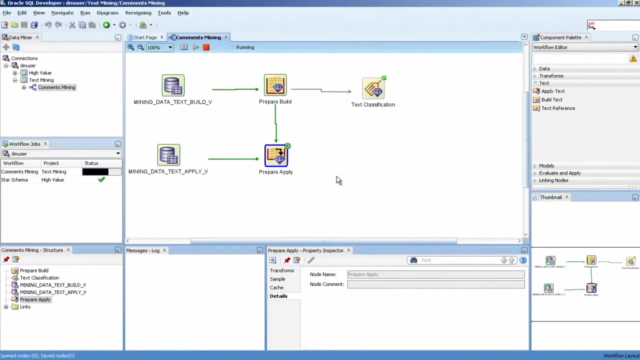 Connect the Prepare Build node to the Prepare Apply node. Connect the Prepare Build node to the Prepare Apply node. Run the node If a Mining Data And If a Mining Data And Select this node to apply the AI test node. It réregulars output data to my memory. 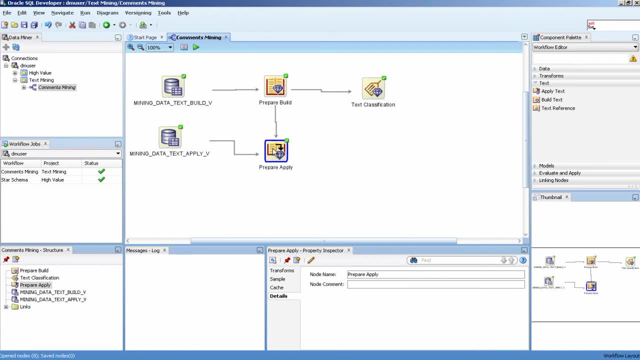 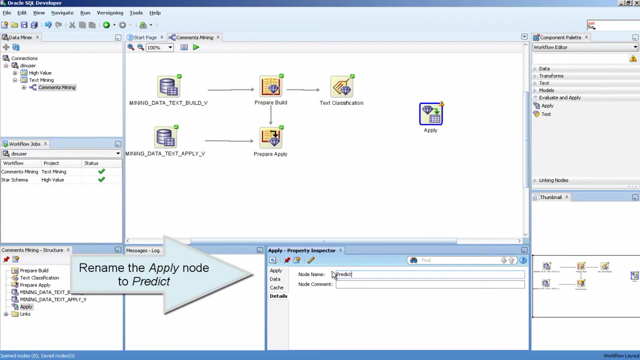 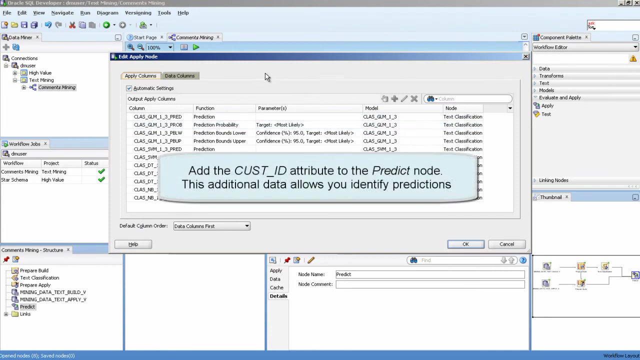 Select the font I mean desired. Select your Shark, A child to呼fte ww2 vai. Add an apply node. Rename the apply node to predict. Add two links to the predict node. Right click predict and select edit. Add the cust id attribute to the predict node. 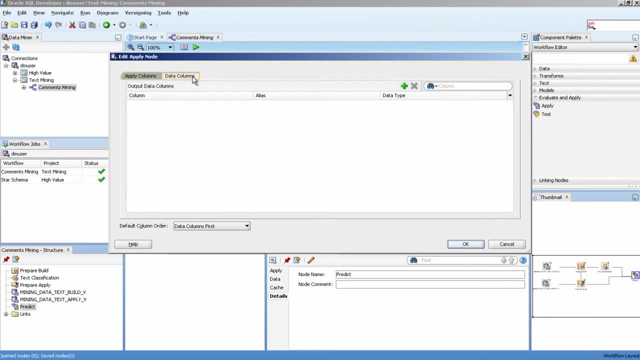 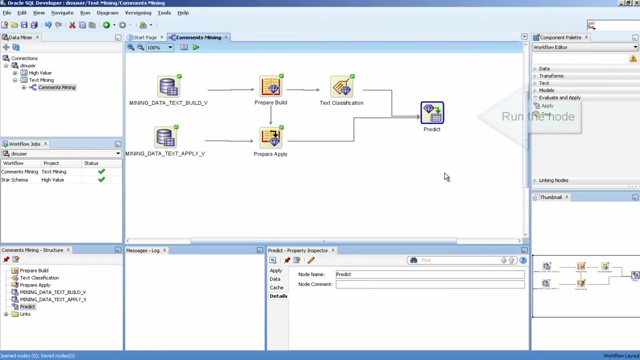 This additional data allows you identify predictions. Add the cust id attribute to the predict node. This additional data allows you identify predictions. Add the cust id attribute to the predict node. Run the node. Here is the data of the predicted node: Run the node. 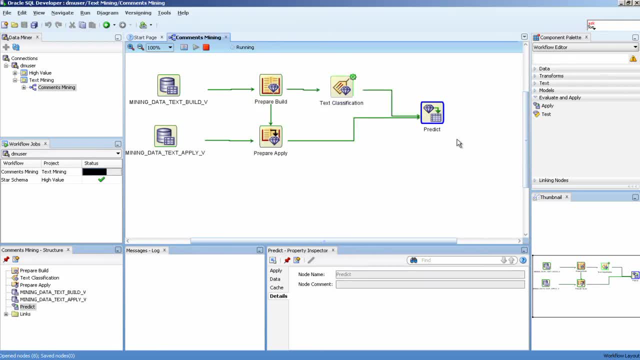 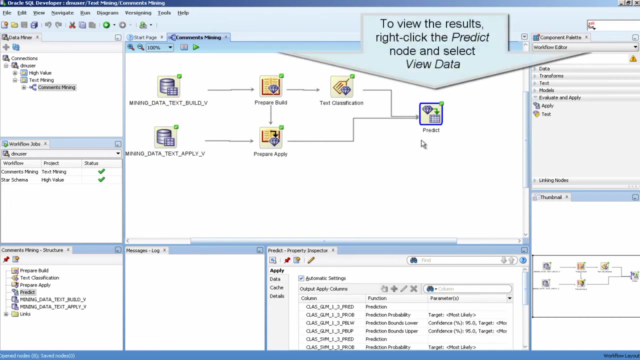 Here is the data of the predicted node. Run the node. Here are the predictions for the predicted node. Press enter to save. Press enter to save the project. Let's run a test. Let's go. Let's run a test. To view the results, right-click the Predict node and select View data.